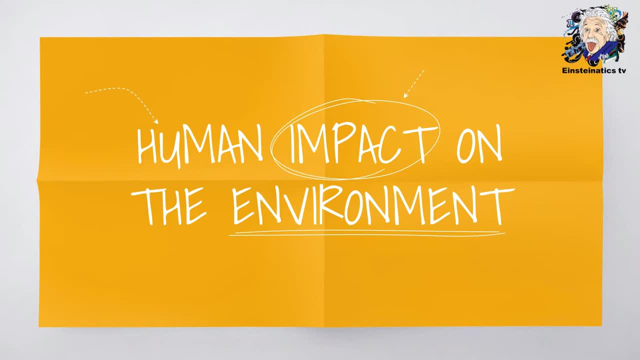 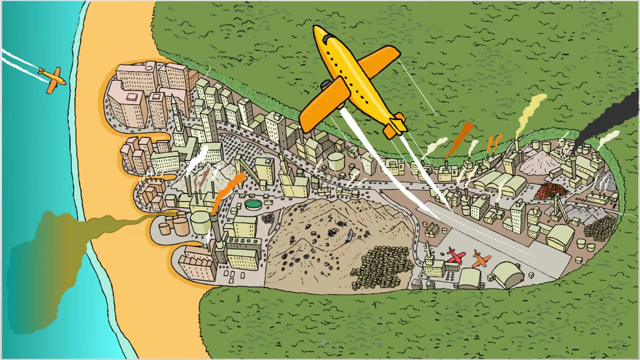 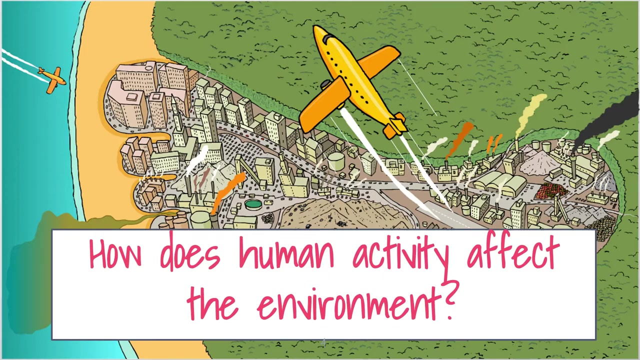 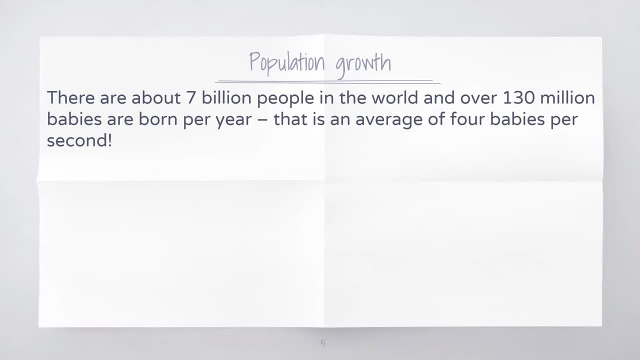 How does human activity affect the environment? The main concern is yung population growth, or yung pagdami ng population ng tao. Just imagine: meron na ngayong 7 billion tao na nabubuhay dito sa mundo and over 130 million. 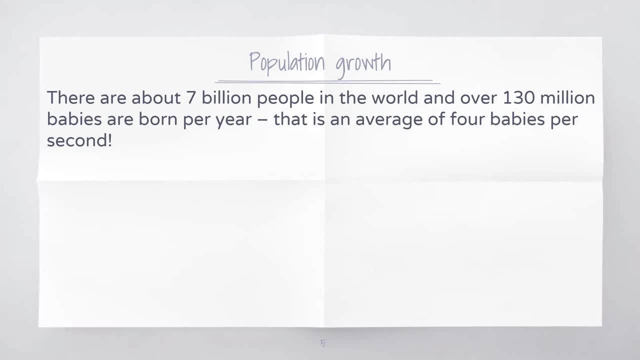 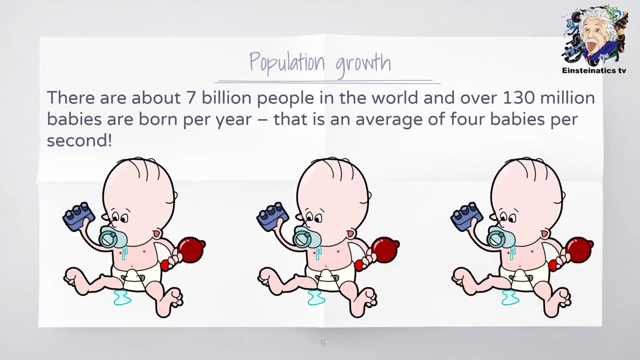 babies ay ipinapanganak bawat taon, So in average that would be apat na baby bawat segundo. So ganun karami yung nadadagdag sa population ng tao dito sa mundo. 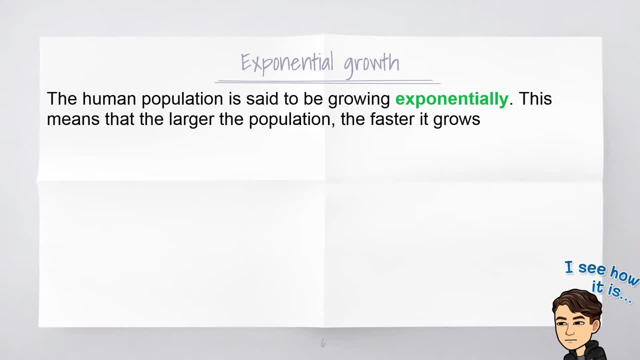 Kung titingnan natin yung population ng tao, we are experiencing exponential growth. When we say exponential growth, ito yung mabilis na pagdami ng population. On our past lessons, we have discussed about carrying capacity and limiting factors. 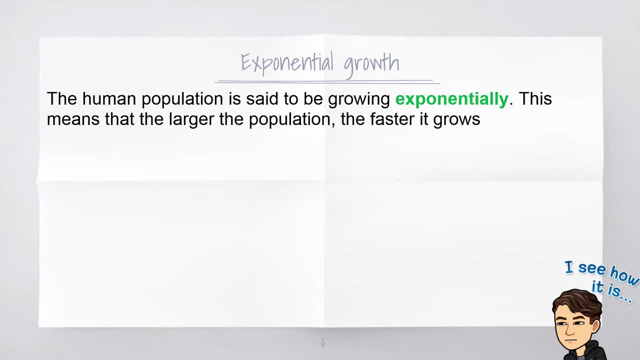 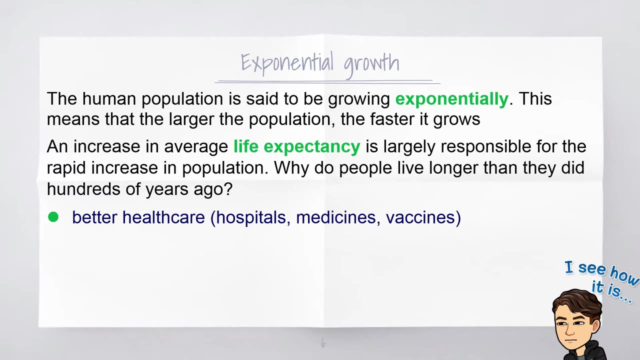 Why do you think that the human population continues to grow despite of these limiting factors? Anyone who care to answer Yes. The reason is that we have better healthcare, meaning we have access sa hospitals, medicines and vaccines. We have also more and better food because of agriculture techniques. 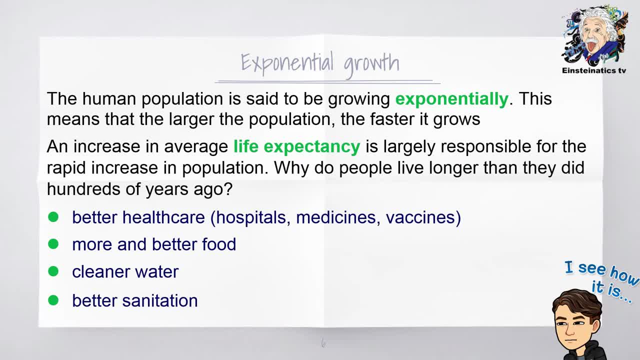 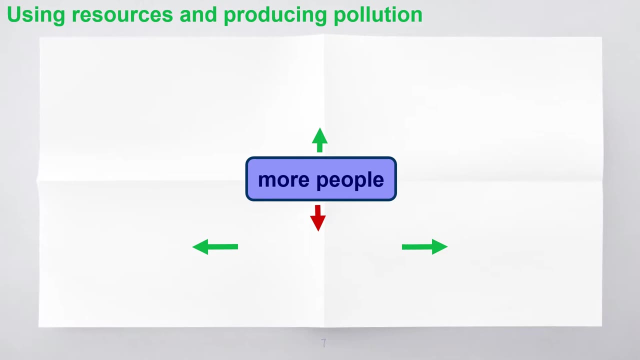 We have also cleaner water and we have better sanitation. So this and all other factors combined, this is the reason why, although meron mga limiting factor, we still have exponential growth. So bakit ba naging concern yung exponential growth ng human population? 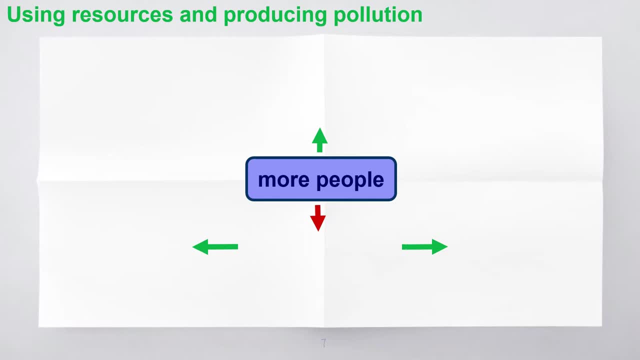 So more people would result in using resources and eventually produce pollution. So pag mas madami yung tao, of course mas marami yung gagamit ng mga raw materials such as the minerals. Or pag mas madami yung raw materials, of course mas marami yung gagamit ng raw materials. 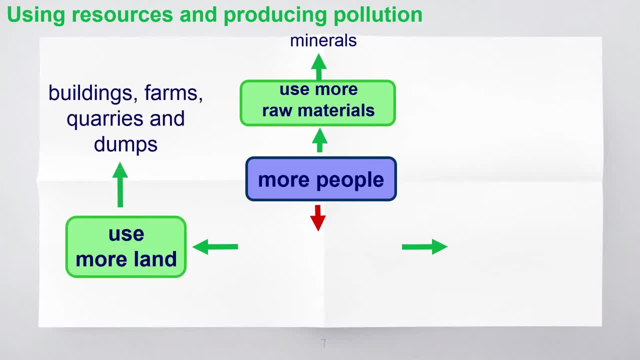 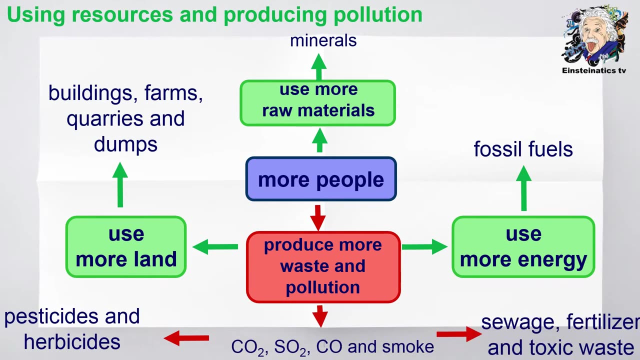 Of course gagamit tayo ng mas maraming lupa to build farms, buildings, quarries and dumps. We also utilize more energy, which we get from fossil fuels, And of course, mas madaming tao. that would also result in production ng mas maraming mga waste products atsaka ng pollution. 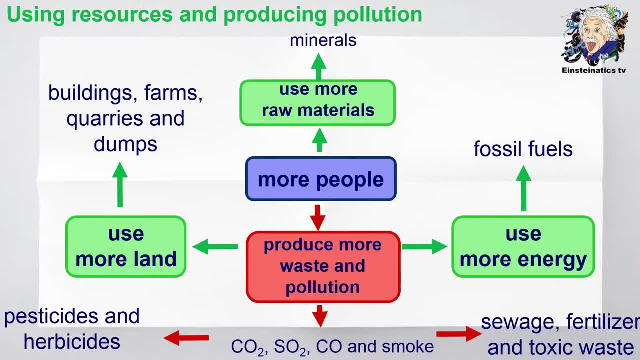 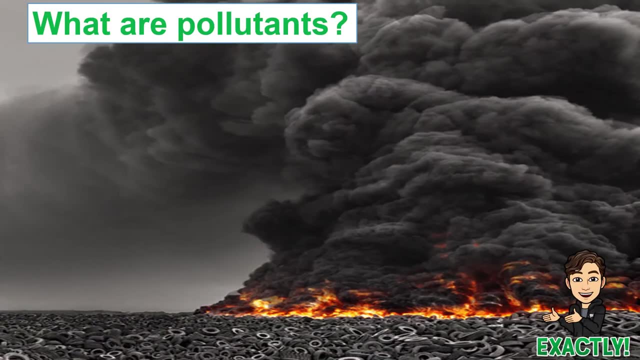 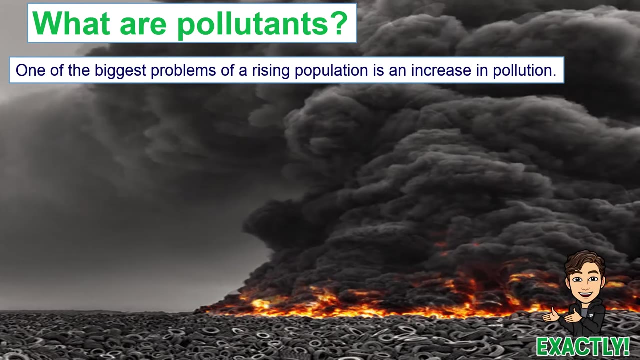 And with this also comes carbon dioxide, carbon monoxide and smoke, which is released using pesticides and herbicides and, of course, through sewage, fertilizer and toxic waste. One of the biggest problem of rising population is yung pag-increase din ng pollution. 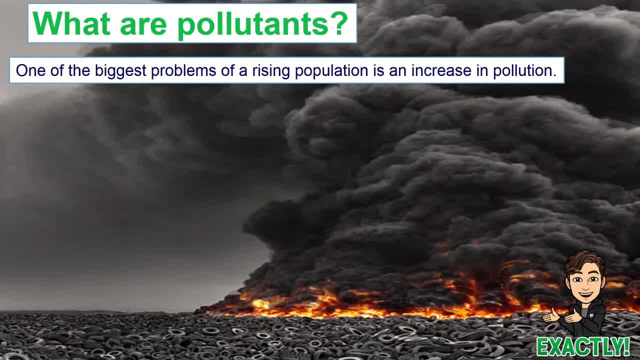 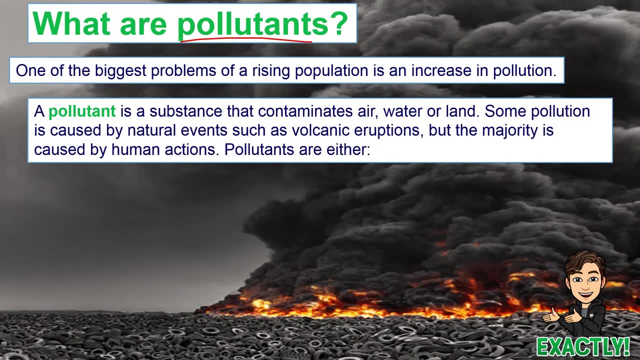 But before that one, it would be better if we would define the term pollutants Pag sinabing pollutants, ito ay any substance that contaminates or nakakadumay sa hangin, sa lupa atsaka sa tubig. 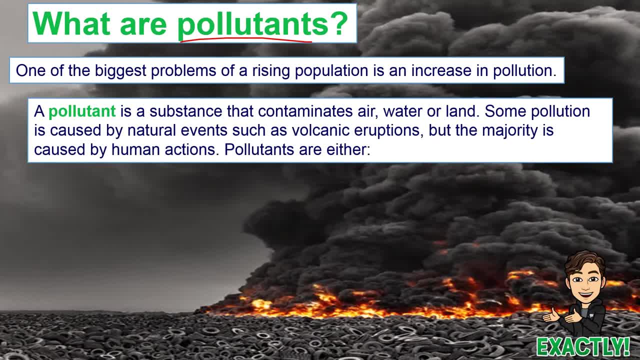 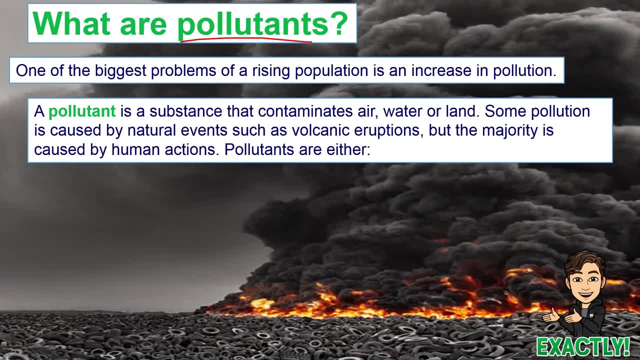 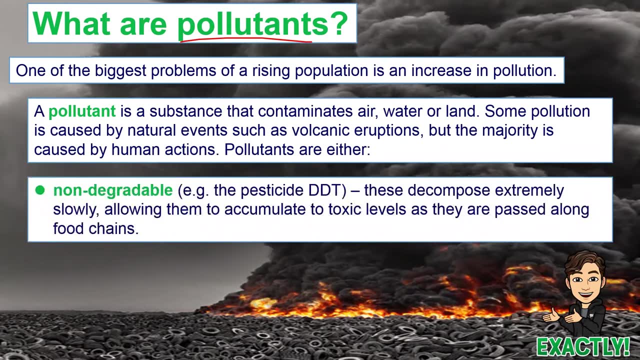 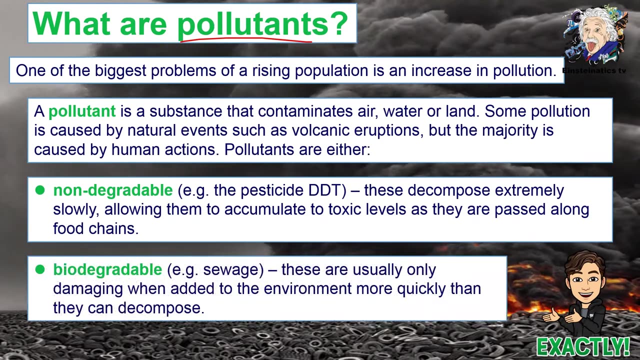 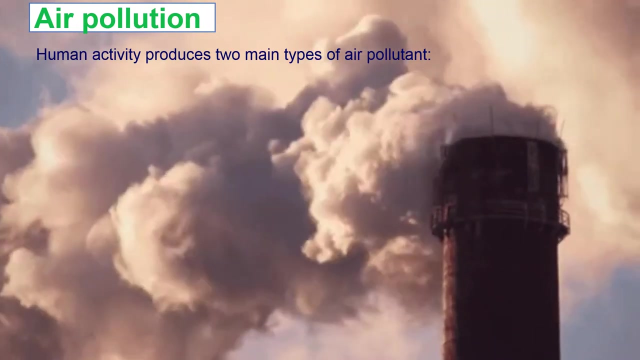 Yung ibang pollution ay pwedeng mag-cause by natural events such as volcanic eruptions, pero karamihan dito yung pollution nag-originate sa human activities. Imano kirana- Click Subscribe. Sif efectos kgena. 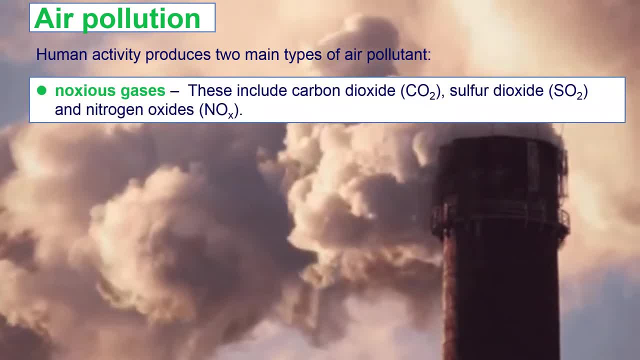 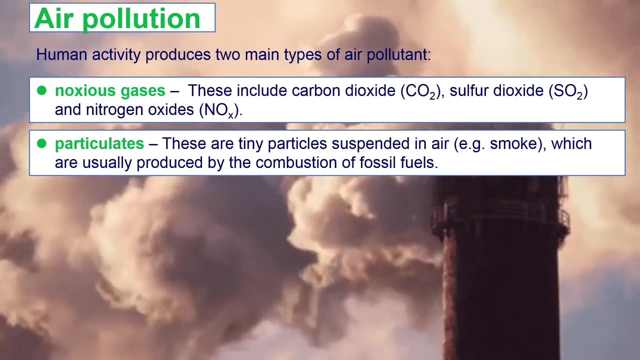 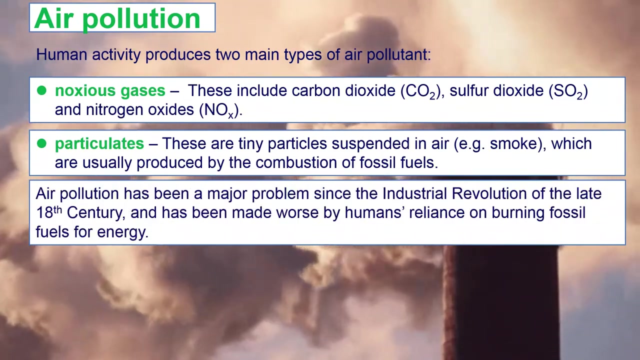 Congratulations, Imano, Congratulations, Go Ahead. I don't want to overthink it, baby, and trick myself back to spite. don't wanna overthink it, baby. it's just me, you're mine, it's them mine. baby, you got me, I ain't fine. 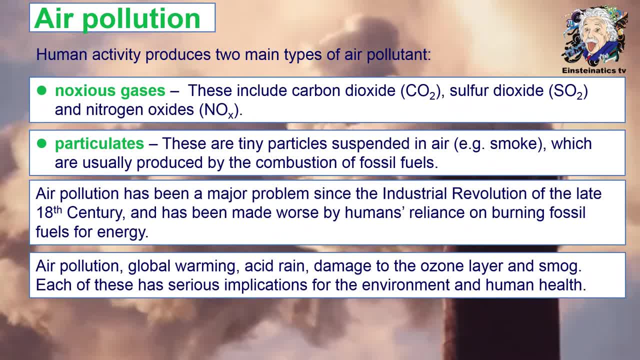 Problemas sa hangin, kabilang yung air pollution, global warming, acid rain, damage to the ozone layer, atsaka smog and lahat ng to ay merong serious implication or masamang efekto sa kalusugan, pati na rin sa kapaligiran. 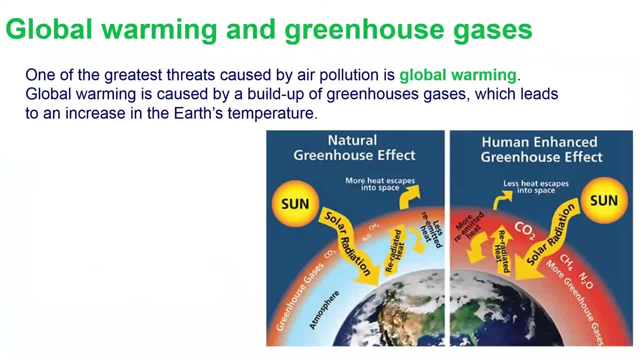 Yung isa sa pinakamalaking panganib na dala ng polusyon sa hangin ay yung tinatawag na global warming. So yung global warming is naidudulot ng build up or pagdami ng mga greenhouse gases. 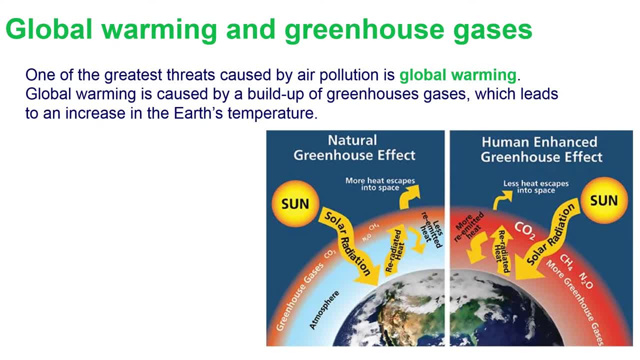 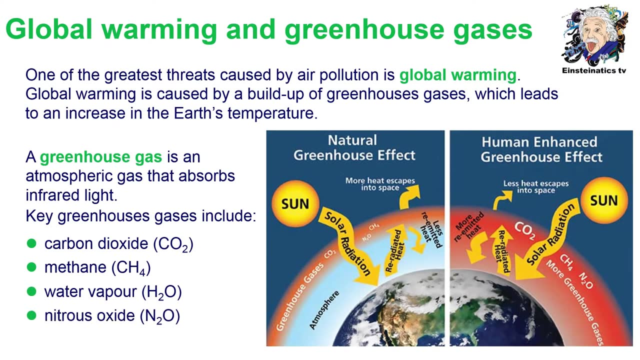 na would lead to pagtaas ng temperatura sa mundo. Ano nga ba yung mga greenhouse gases. So, yung mga greenhouse gases, yung mga greenhouse gases, yung mga greenhouse gases, yung greenhouse gases na tinutukoy is yung carbon dioxide, yung methane, water vapor and of. 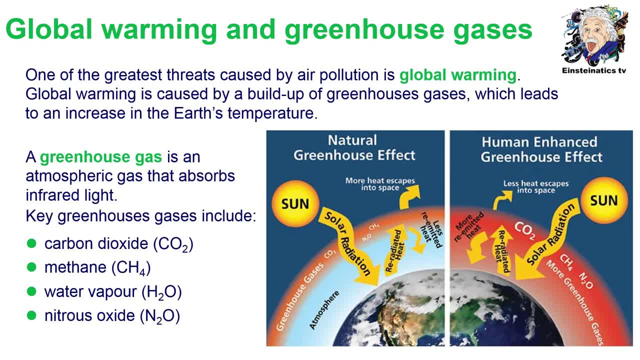 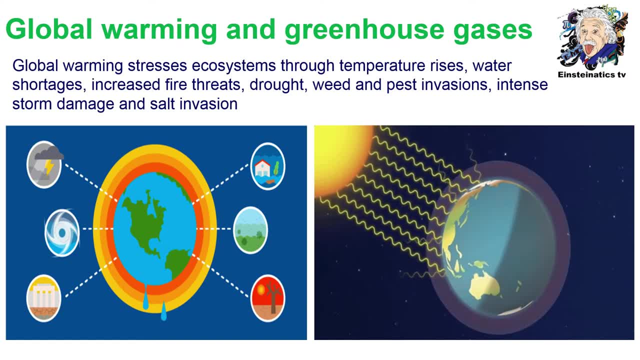 course, yung nitrous oxide. So why do we need to worry on global warming, atsaka sa greenhouse gases? It is for the reason that global warming stresses ecosystems or naapektuhan tayo nito, dahil sa patuloy na pagtaas ng temperatura. 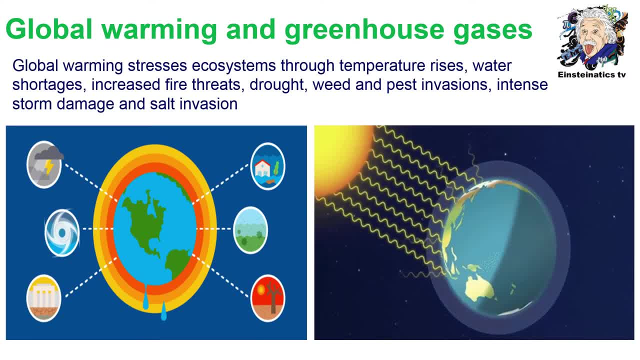 That is the reason why nagkakaroon ng greenhouse gases, Ang kakulangan sa tubig mas marami yung mga fire threats, kagaya ng pagkasunog ng mga forest, yung tagtuyot, yung weed and pest invasions, not to mention. this is also attributed kung 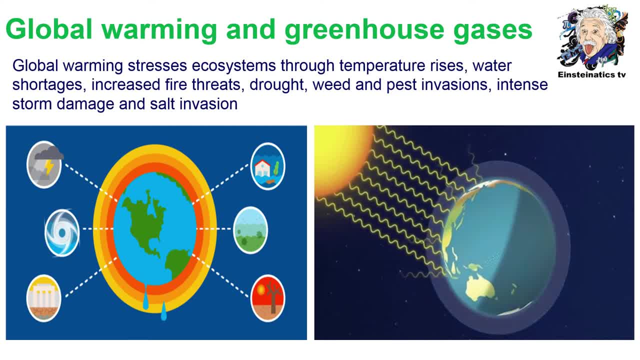 bakit sa bawa taon mas marami yung bagyo at mas lumalakas yung mga bagyo na nararanasan natin. It also is attributed why the polar ice caps are melting and that is why there is an increase. 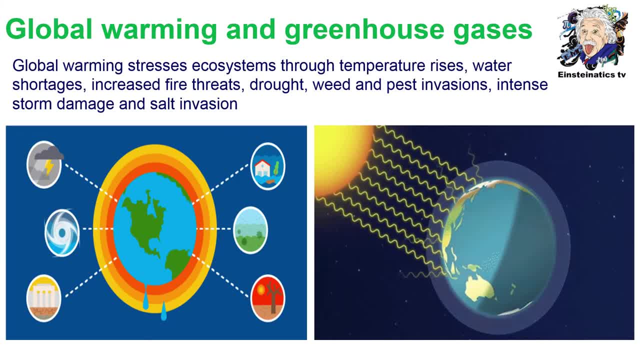 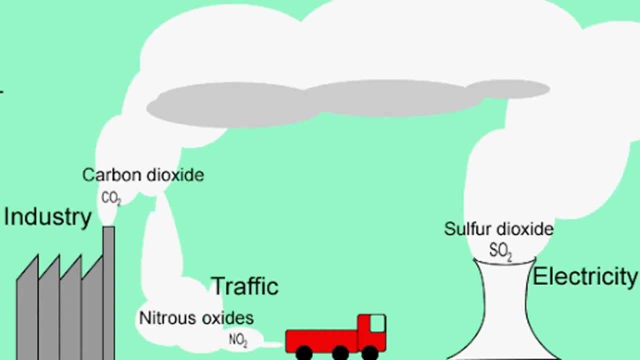 in the sea level and that is why yung ibang mga isla ay unti-unting lumulubog, and, of course, yung salt invasion because of the increased water level. Another adverse effect or masamang epekto ng air pollution is yung tinatawag na acid rain. 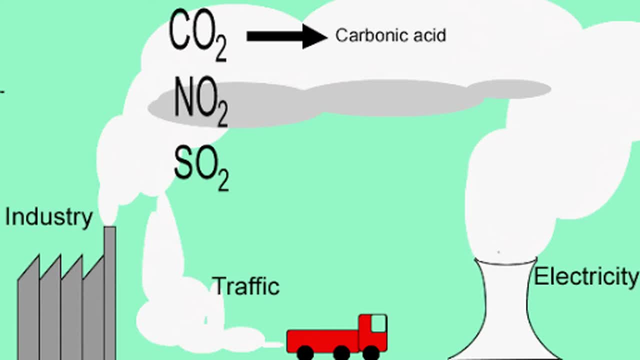 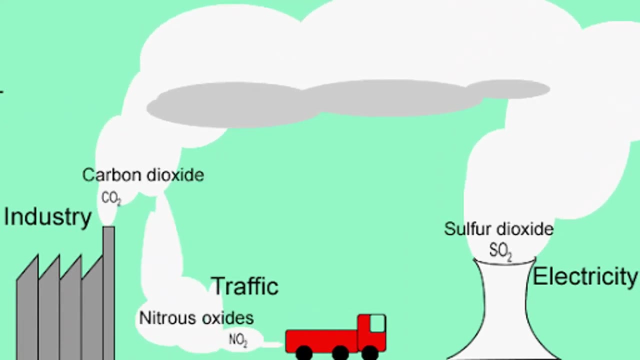 Yung acid rain is nag-o-originate dahil sa dependency natin sa paggamit ng fossil fuels as source of energy. So ito lang nanggagaling sa usok na binubuga, galing sa pabrika sa mga sasakyan, pati na rin yung source of energy natin, pag produce ng electricity. 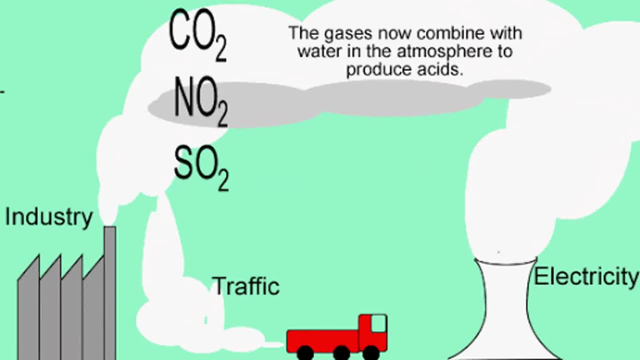 So yung carbon dioxide, nitrous oxides, pati na rin yung sulfur dioxides. ito ay nagsasama-sama and would form now into acids, which now falls back to earth. Ano nga ba yung efekto nito. 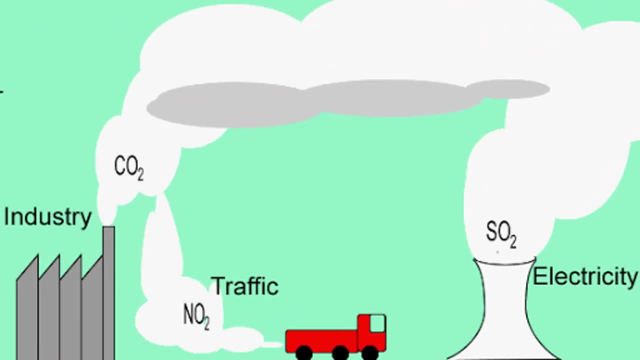 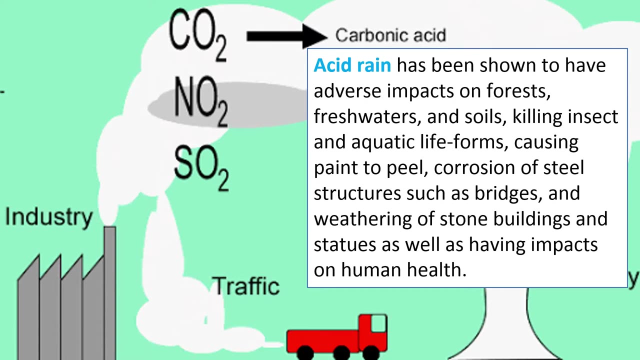 Once na it would fall back down to earth. Ano nga ba yung efekto nito? Once na it would fall back down to earth. back down to earth as an acid rain. Based on study, it has a bad effect on forests. 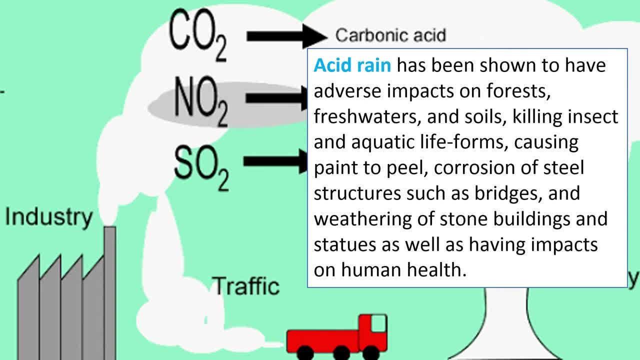 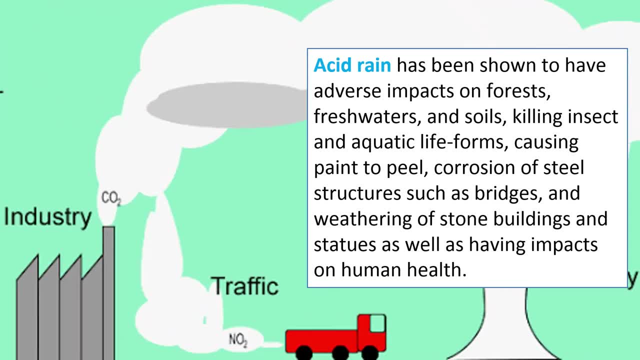 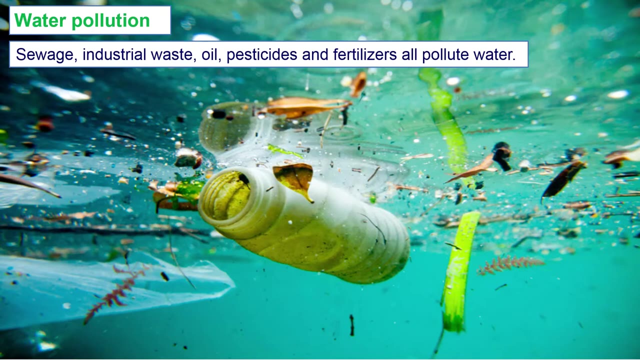 freshwater and land. It kills all kinds of insects and aquatic life forms. It also causes pain to peel, corrosion of steel structures such as bridges, weathering stone buildings, and also has a bad effect on human body. Another type of pollution is: 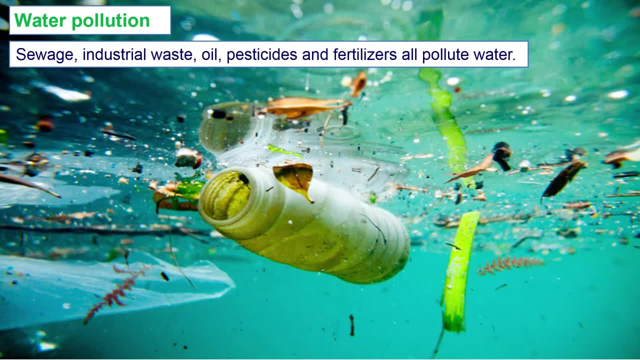 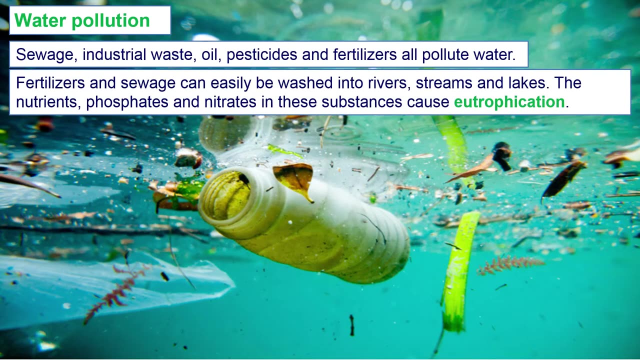 the pollution in water. This happens when the sewage, the cement of the factory and oil, pesticides and fertilizers enters water. Aside from the water becoming dirty, not fit for human consumption, or it becomes unpatable, kasi pwedeng magdulot ng sakit? 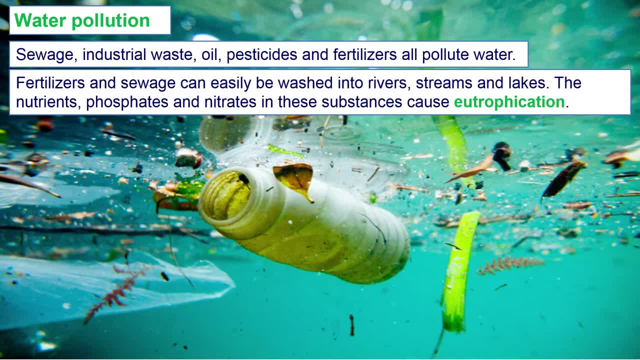 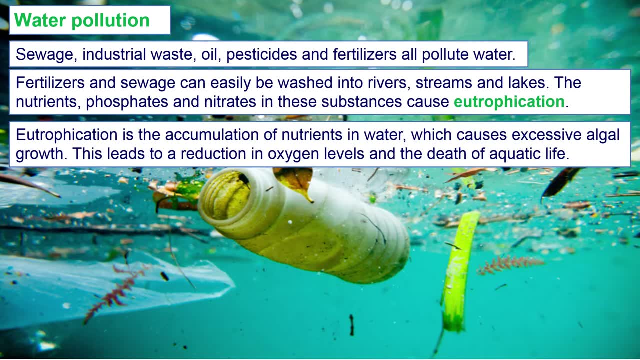 another effect of water pollution is yung tinatawag na eutrophication. Ano nga ba yung eutrophication? Yung eutrophication ay yung biglaang pagdami ng mga nutrients sa tubig na. 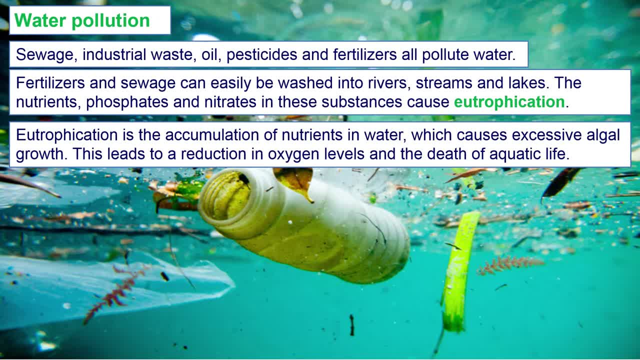 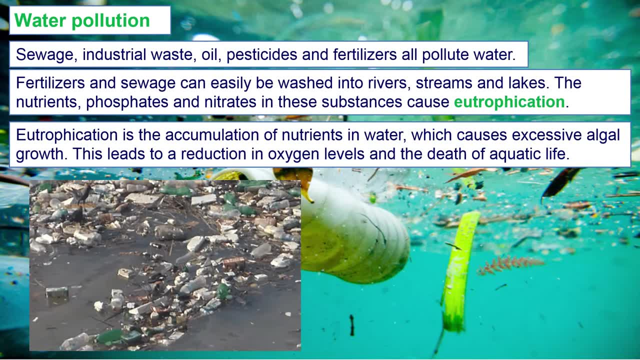 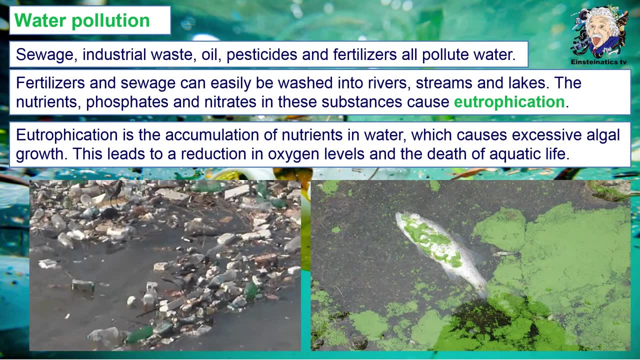 ito ay magdudulot ng maraming pagtubo or excessive growth of algae, and ito ay magdudulot ngayon ng pagkaubos or pagbaba ng oxygen level, na magdudulot naman ngayon ng pagkamatay ng aquatic life. 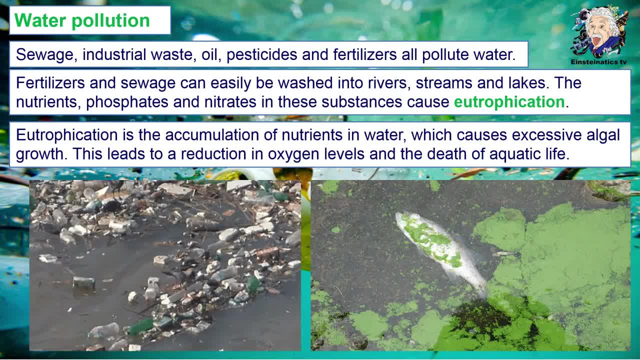 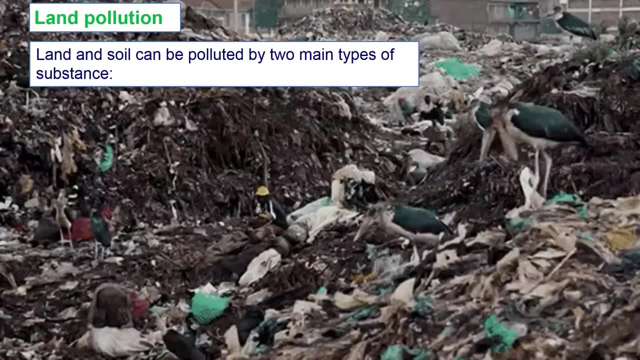 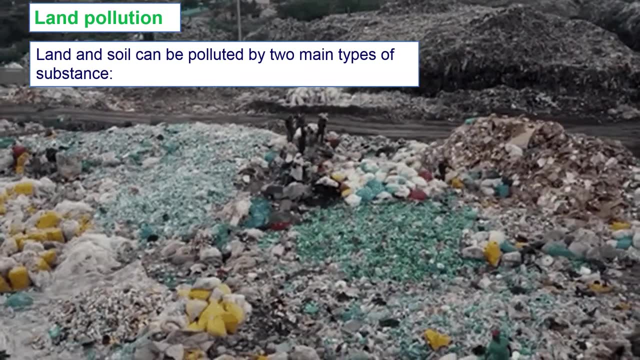 kagaya ng mga isda, kasi wala na silang pagkukunan ng source of air. The last type of pollution is yung pollution sa lupa. Yung lupa or soil ay pwedeng ma-pollute sa dalawang paraan or dalawang main. 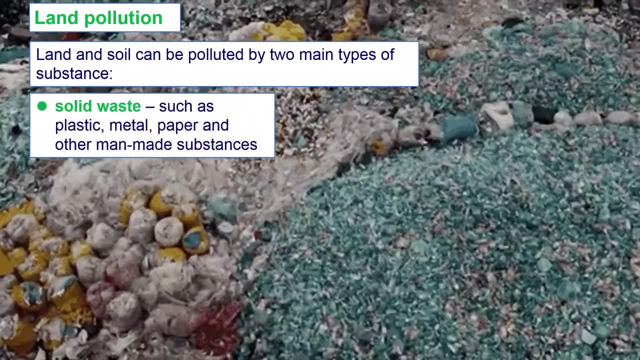 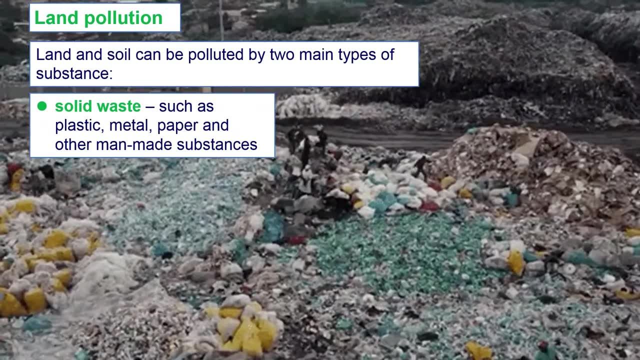 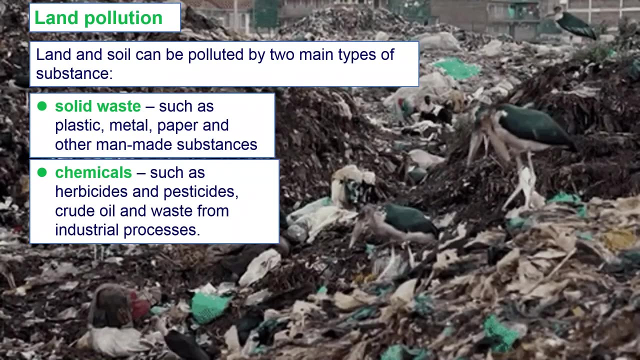 substance Yung una is yung tinatawag na solid waste, So kabilang na dito yung mga plastic, yung mga metal, yung paper at kung ano pa mang mga man-made substances. Yung ikalawa naman is pwedeng itong ma-pollute through chemicals such as herbicides and pesticides, crude oil at saka yung mga waste from industrial processes. 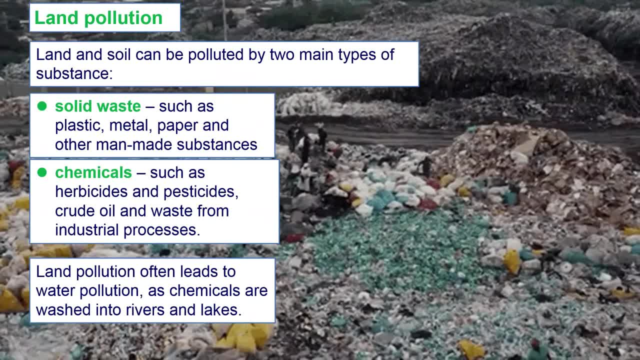 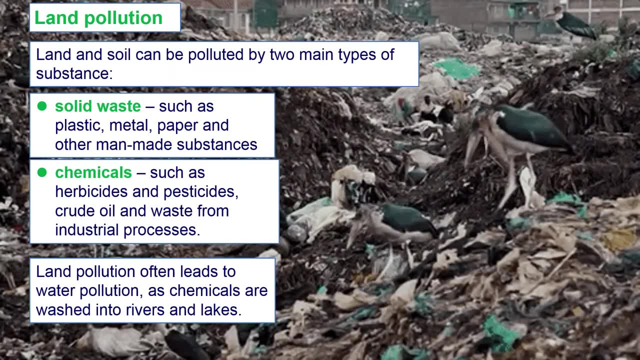 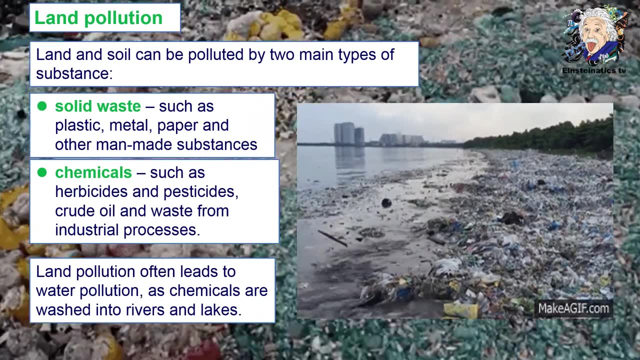 So yung land pollution often leads to water pollution, kasi pag umulan ma-wash out into the rivers and lakes and eventually into the sea. So ayan, that's the effect from land pollution. yung duminag nandun sa lupa ay pwedeng madala doon sa tubig. 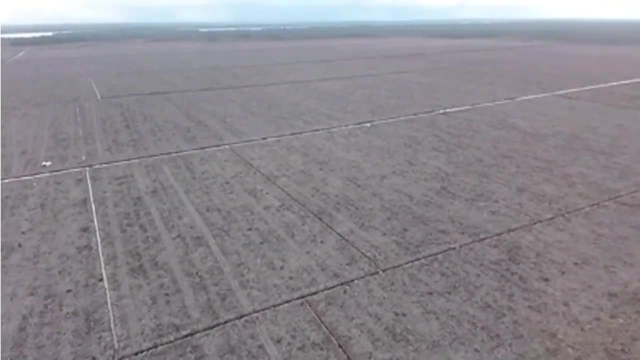 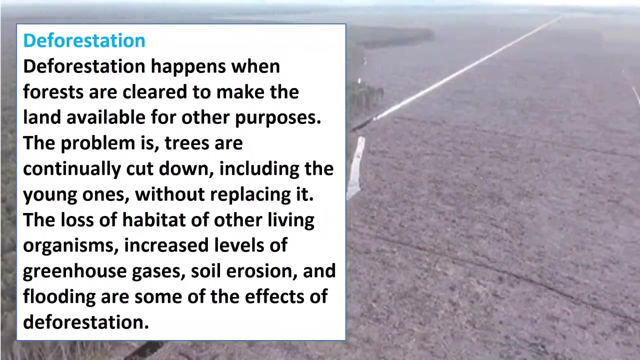 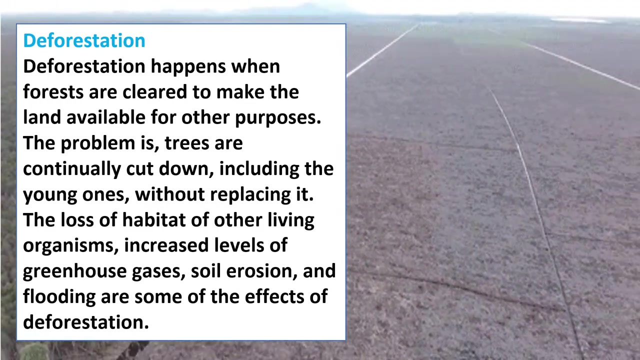 Another environmental issue or concern is yung tinatawag na deforestation. Ano nga ba yung deforestation, Ano nga ba yung deforestation? Yung deforestation ay nangyayari. Yung deforestation ay nangyayari pag yung kagubatan ay being cleared to make land available for other purposes. 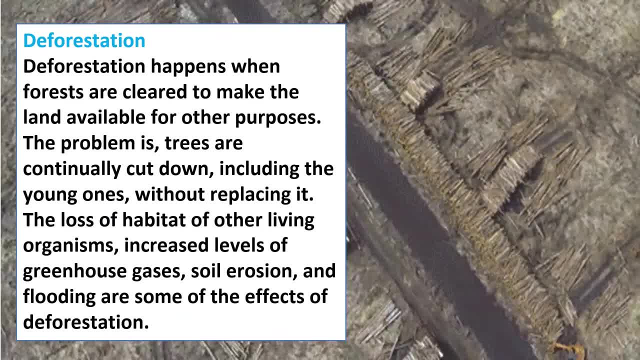 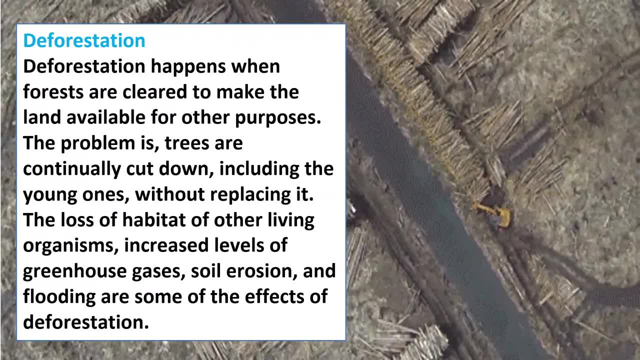 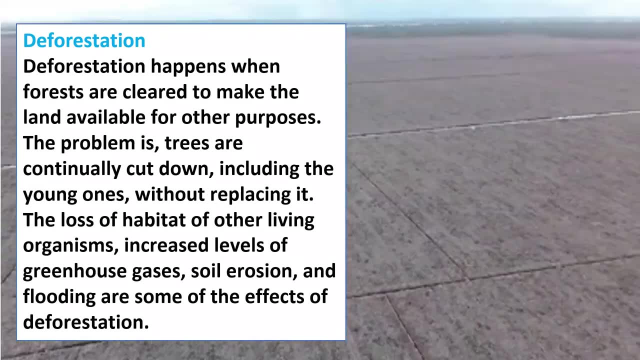 Yung nagiging problema dito is yung mga puno na pinuputol, kabilang na rin yung mga maliliit pa ay hindi napapalitan. As an effect, nawawalan ngayon ng tirahan or habitat yung other living organism and there would be an increased level of greenhouse gases, soil erosion and flooding. 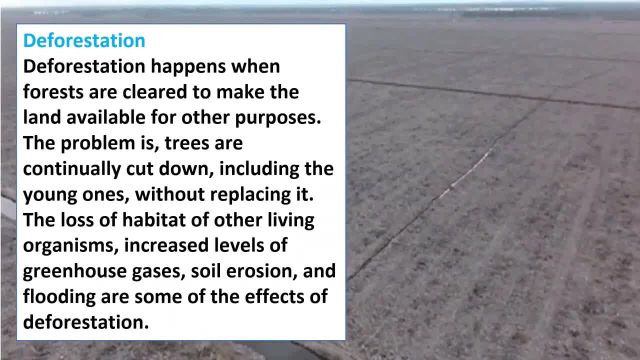 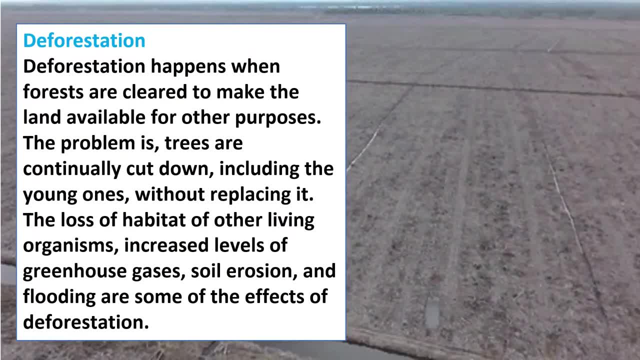 Or some of the effects of deforestation, which is very evident now sa naranasan ng ating bansa due to typhoon Ulysses, Dahil sa mining and large scale deforestation doon sa mga lugar na binabaha. 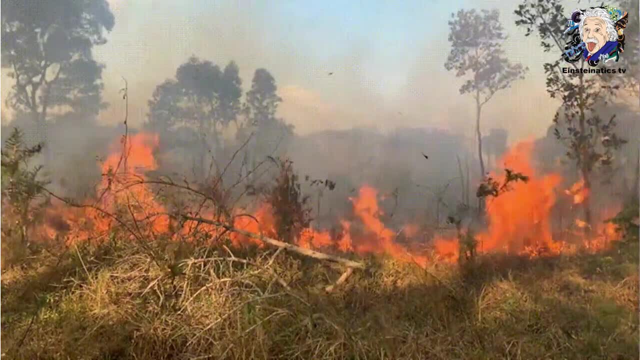 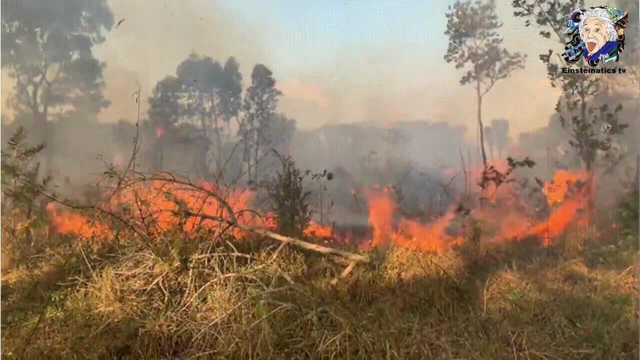 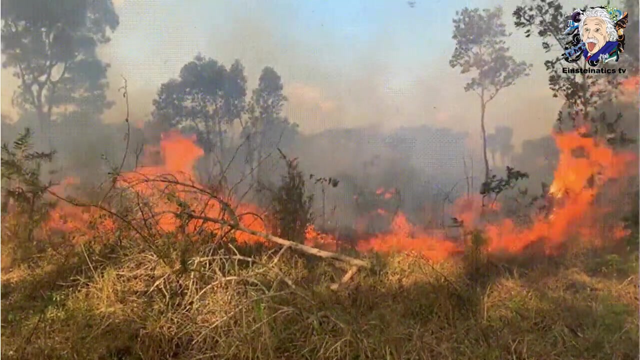 Now another bad practice na observable dito sa Pilipinas is yung tinatawag na kaingin system which, in order for the farmers to create a fertile farmland, is sinusunog nila yung mga bushes, yung trees, at yun yung tinatawag na. 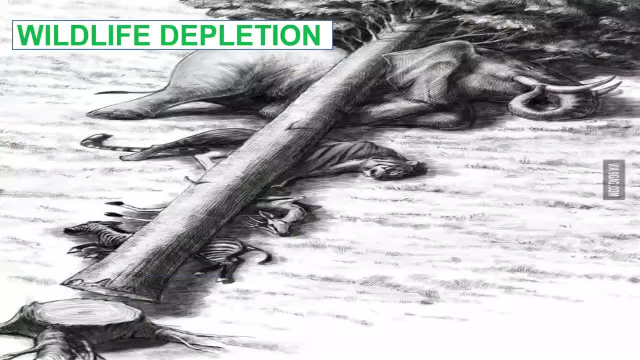 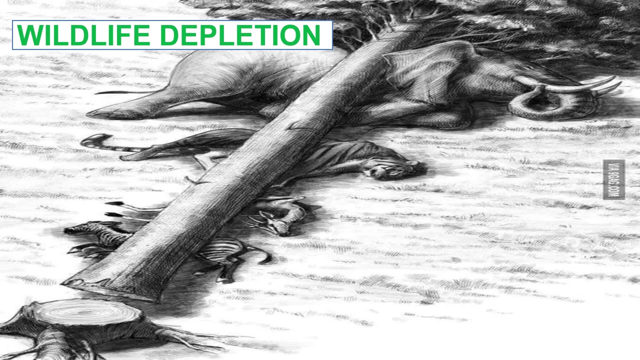 kaingin system. the next environmental issues and concern that we would be discussing is about wildlife depletion. ano nga ba yung wildlife depletion? do you have any idea? as what the picture clearly shows? ito yung unti-unting pagkaubos ng flora at fauna. 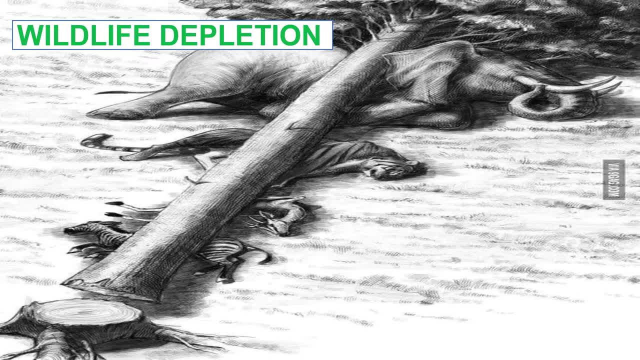 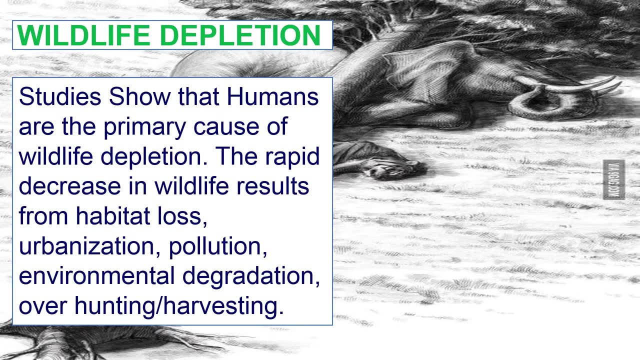 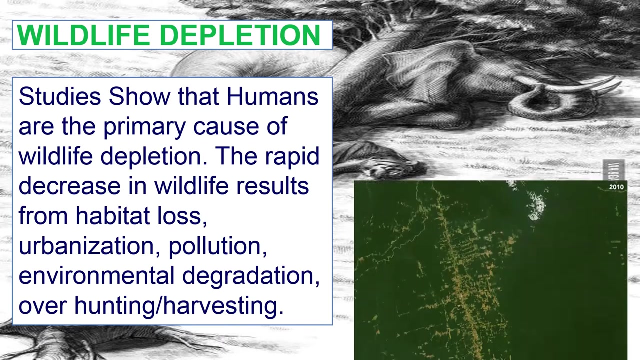 so do you have any idea kung bakit nangyayari ito? yes, studies show na tayo yung biggest reason kung bakit mabilis na nauubos yung wildlife: it is because yung due to habitat loss dahil sa rapid urbanization, yung pag develop ng forest and turning them. 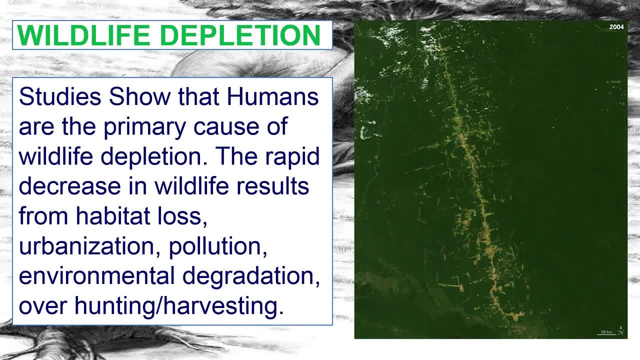 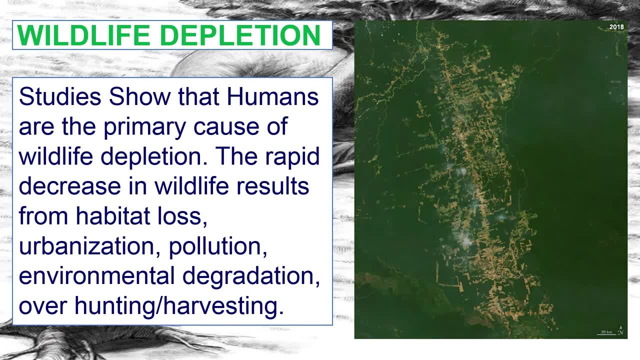 into residential lands or residential places. we have also produced too much pollution, environmental degradation, pati na rin yung over hunting and harvesting. if you are going to look at the picture on the right, you could clearly see from 2001 to 2009 yung nilang. 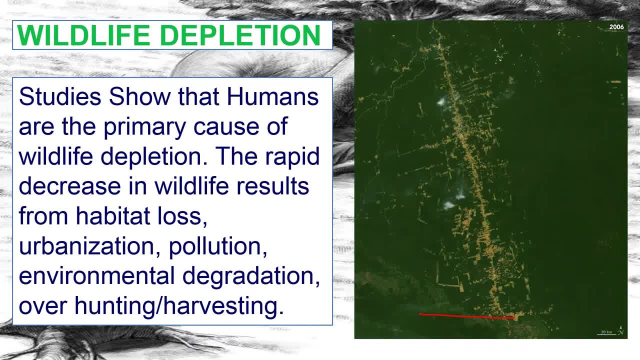 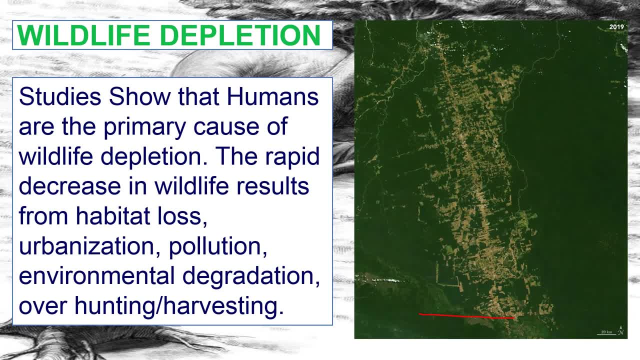 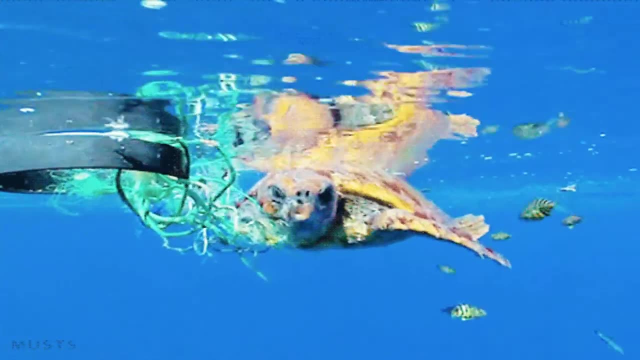 19, kung paano na-develop or unti-unting nababawasan ngayon yung flora at saka fauna ng Amazon Forest Ayan being converted for human usage. The type of environmental issue and concern that we would be dealing is the destruction. 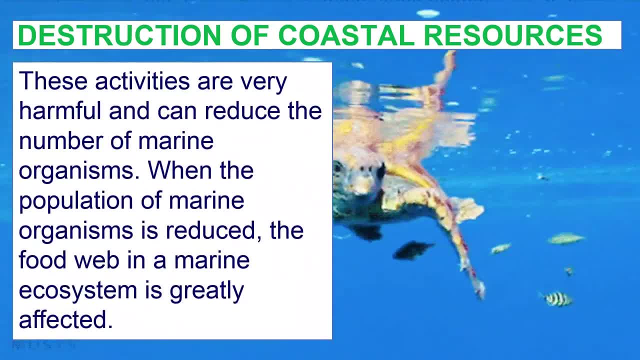 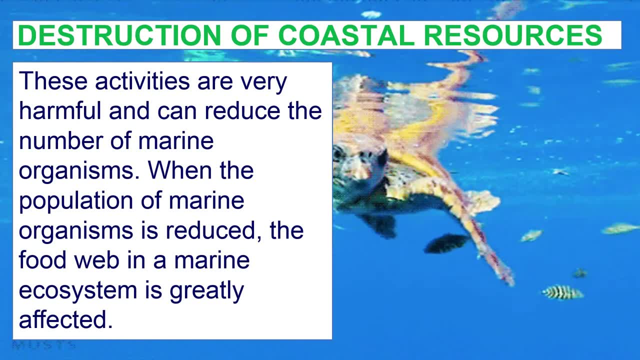 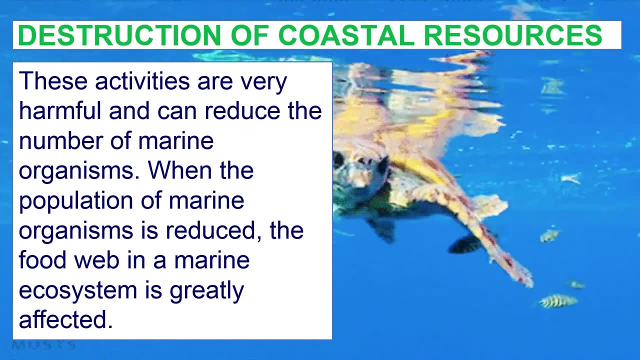 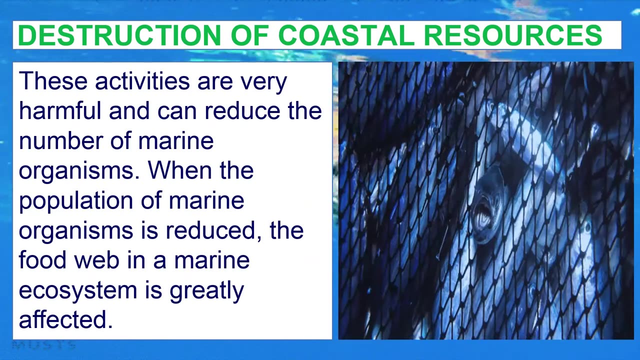 of coastal resources, There are a number of activities na pwedeng makasira sa ating marine life. When the population of marine organisms is reduced, the food web in a marine ecosystem is greatly affected. Ano nga ba yung human activities na may masamang nadudulot sa ating marine resource? 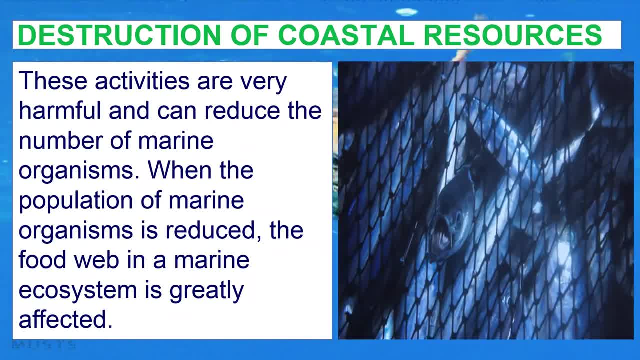 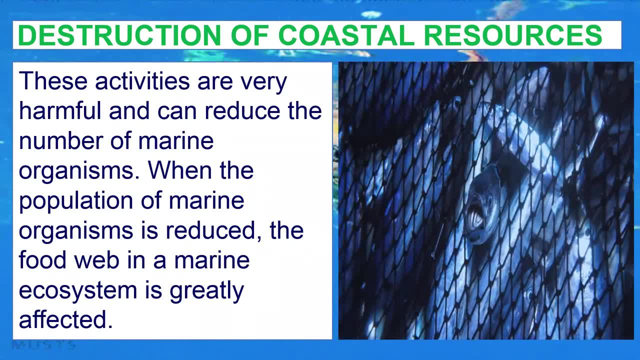 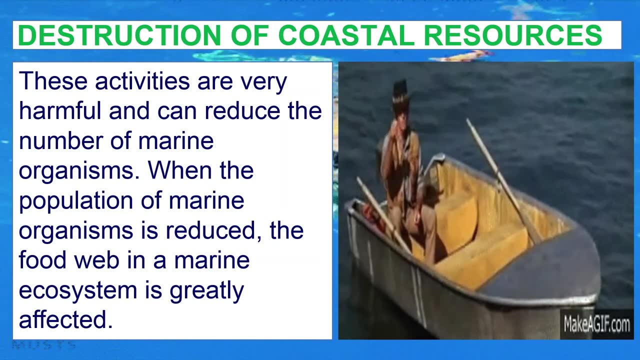 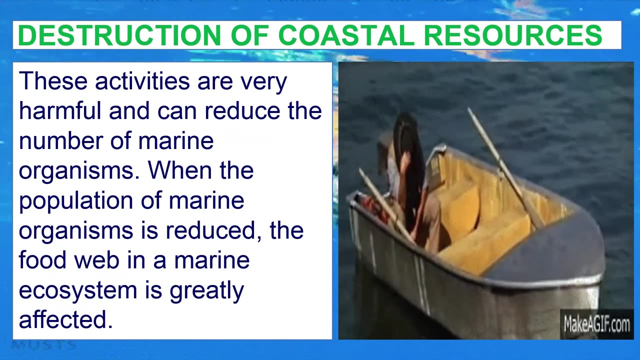 Yung una dyan is, of course, yung overfishing, Yung consumption ng tao Is nag-i-increase because of our increase in population. Another bad practice is, of course, yung dynamite fishing, Na kahit yung mga malilit na isda is namamatay dahil sa method na to. 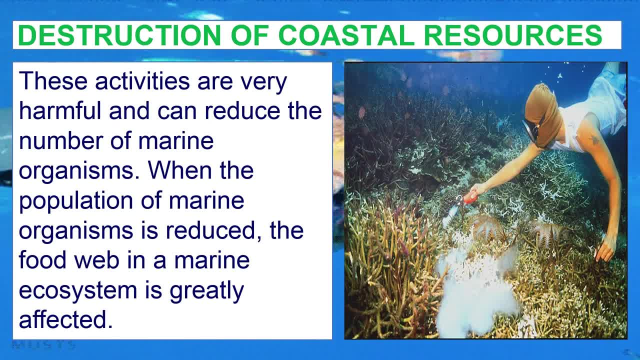 Another human activity that destroys our coastal resources is yung tinatawag na cyanide fishing. Ano nga ba Yung cyanide fishing? Ito yung paggamit ng chemical na cyanide para manghuli ng mga aquarium fishes. 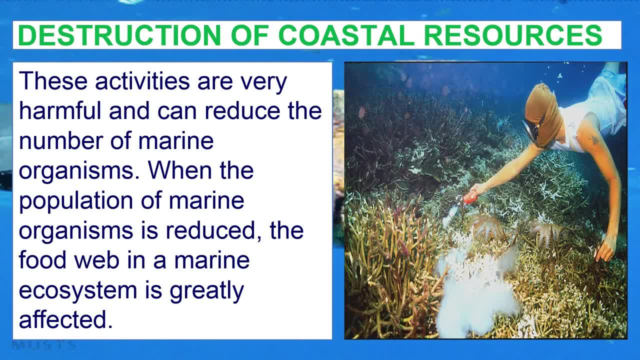 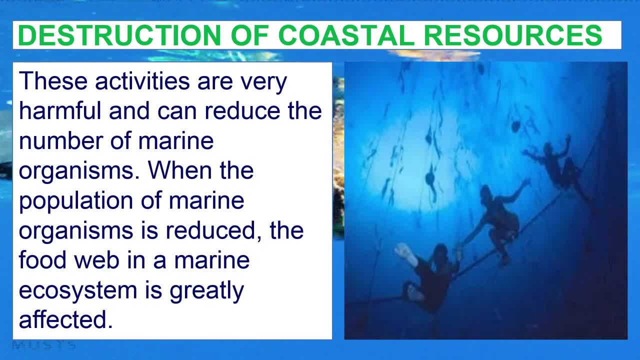 Now this would in turn, harms the coral reefs or destroys it. Yung another bad fishing practice is yung tinatawag na moroami. Yung moroami is that yung mga fishermen ay gumagamit ng mga bato para sirain yung corals. 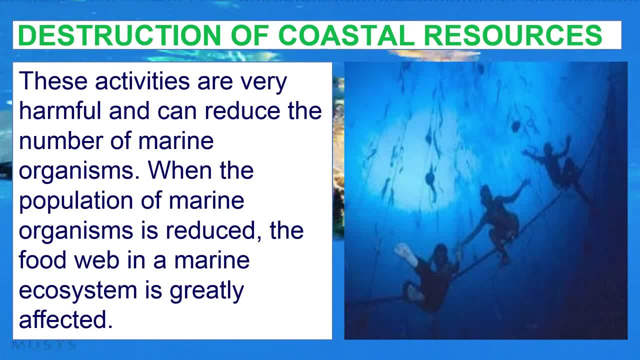 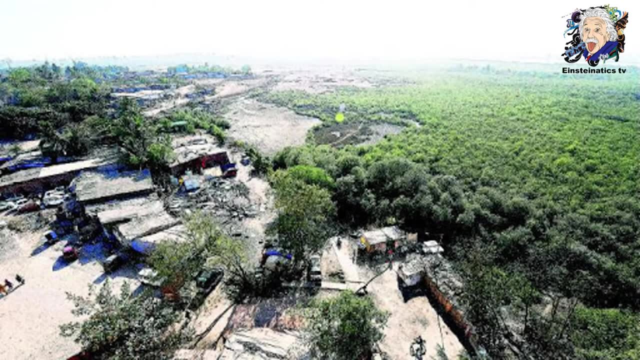 para maitaboy yung mga isda papunta dun sa net. And yung another big factor kung bakit rapid yung pagkasira ng ating coastal resources is of course yung encroachment sa mga mangrove areas, pati na rin yung development ng mga seashores into residential areas. 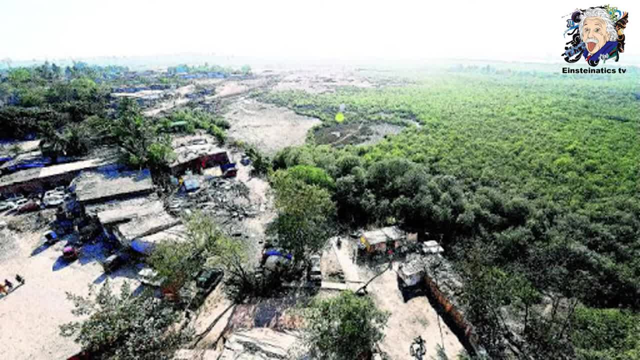 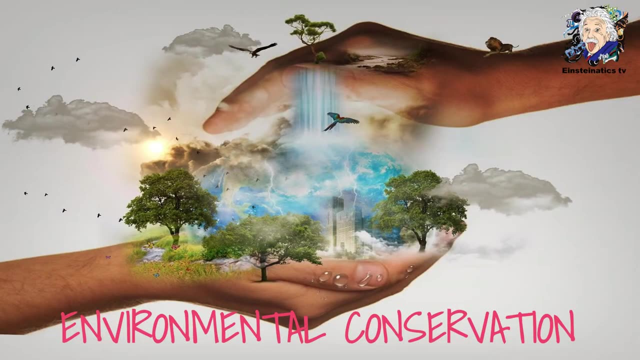 which in turn destroys or sinisira yung natural habitat ng mga organisms na pumapatay ngayon sa mga li- wildlife na nakadepende dito. Now that we are through on the different environmental issues and concerns, this time papag-usapan naman natin kung paano tayo makakatulong. 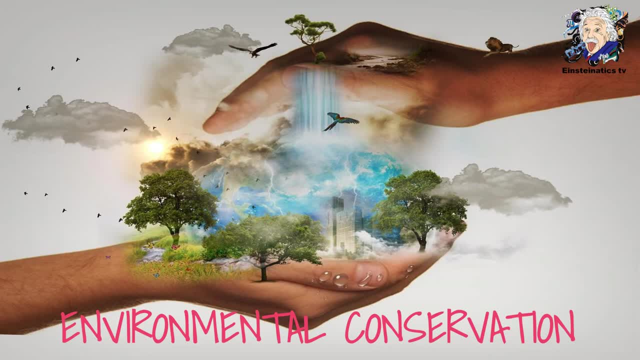 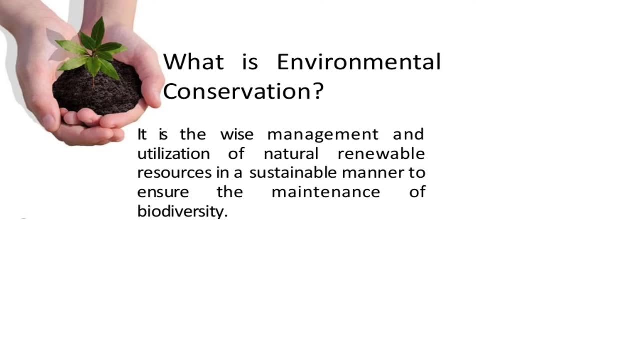 how to do our part in environmental conservation. Ano nga ba ang environmental conservation? Environmental conservation is defined as yung waste management and utilization of natural renewable resources in a sustainable manner to ensure the maintenance of biodiversity. So paano ka nga ba makakatulong in order for you to conserve the environment?